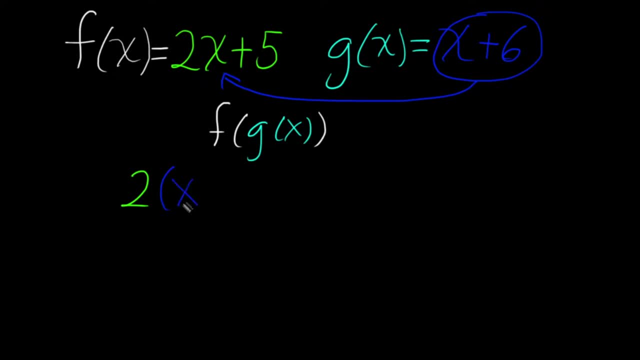 x. this time it's multiplying by the g function, x plus 6, and then we still have the plus 5 after. We'll want to simplify. so this is equal to distributing the 2 in gives us 2x plus 12 plus 5, and finally we'll combine like terms and get 2x plus 17, and that's our final answer for. 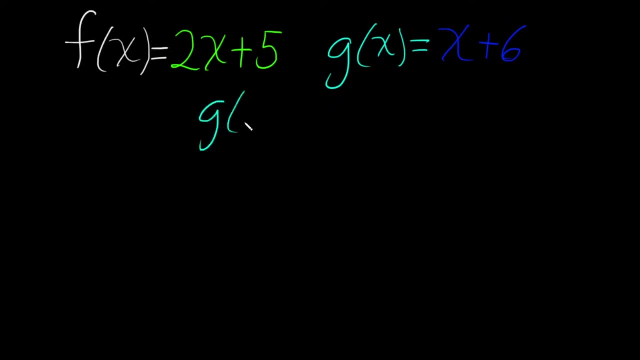 f of g of x. This time let's find g of f of x. Now the f function is on the inside, so we'll have to take this entire function here and plug it in to the x value of the g function. Keep in mind, if 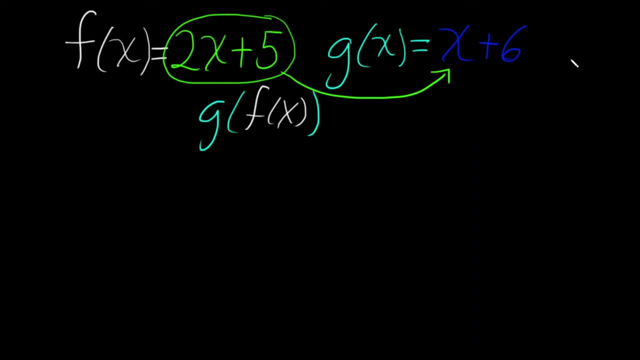 there were multiple x's, then this function would have to replace every single x there is. We have 2x plus 5. that replaced the x here, and then we still have plus 6 afterwards. We'll combine like terms and get a f of g of x. Now let's find g of f of x. This time. let's find g of f of x, Now the f of x. 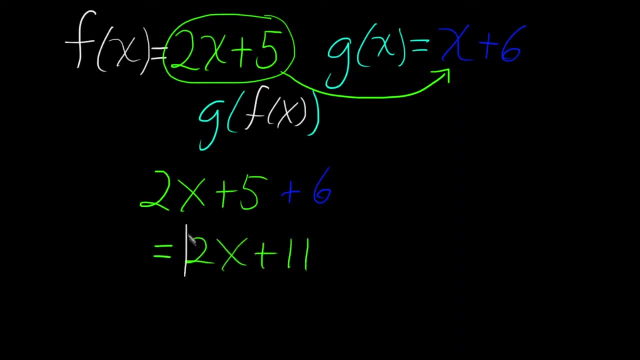 was opposite: g, x plus 5. So we now use almost 1 function per x. here We'll use 16 and get 2x plus 11, and that's our final answer. Let's try these 2 functions. We'll do f of g, of x first again. 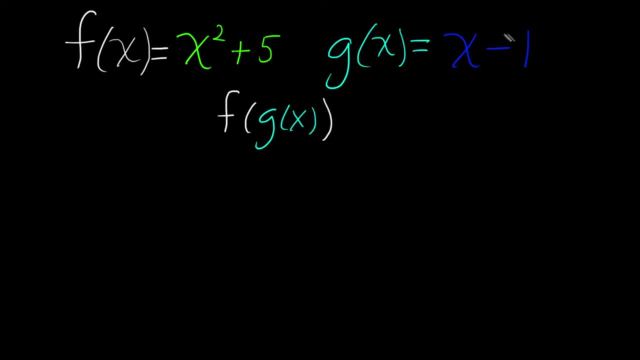 like we saw earlier, g of x is the inside function, so we'll take all of that and plug it in for every x in the f of x function. So instead of just x being squared, we're going to square the entire x minus one, like this: x minus one squared, and then we need to include the rest of the. 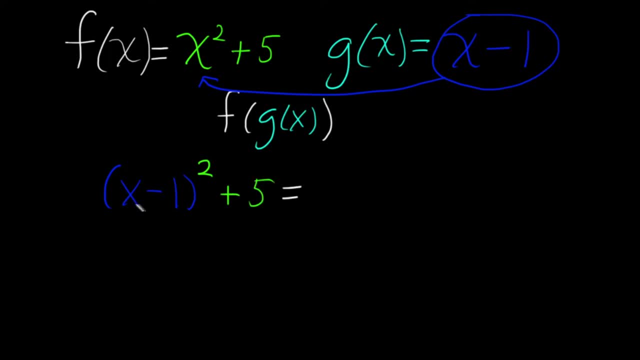 function plus 5.. So we look at that. so we now have 3 equals math, so it's 2 x plus 11, so 1 plus 5.. Here we can start simplifying. Be careful not to distribute the square, because x minus 1 squared. 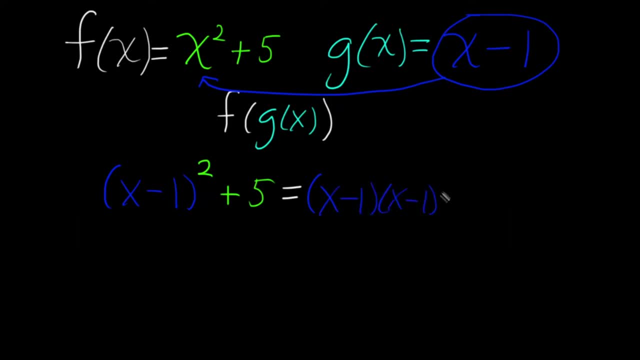 really means x minus 1 times x minus 1.. We still have plus 5.. If we foiled this out, we would get x squared minus x minus x plus 1 and then plus 5.. We'll combine like terms. We have x squared. 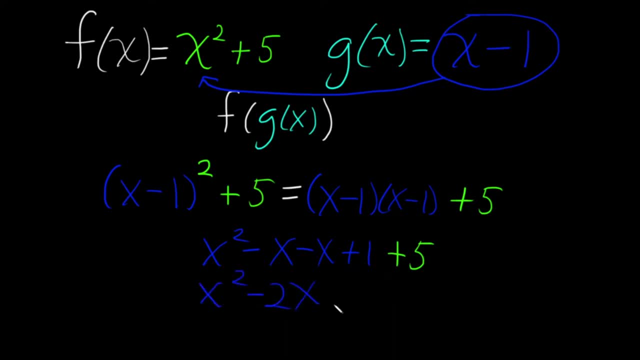 minus 2x, and the plus 1 and plus 5 will combine to plus 6.. And this would be our final answer for f of g of x. Now let's do g of f of x. The f function is on the inside, so all of the f of x.